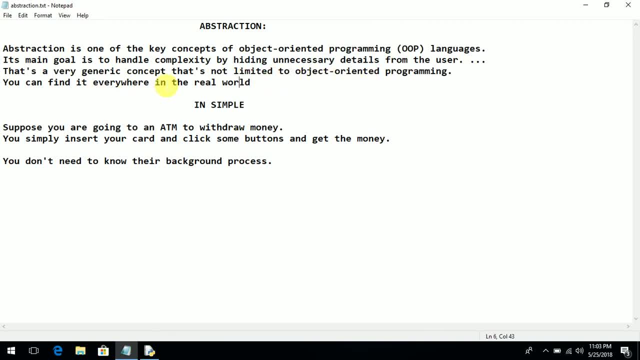 limited to object-oriented programming. You can find it everywhere in the real world. Okay, In simple words, you can say: you can hide unwanted detail from user, Like if user gives you the input, so you have to show them the output. You don't need to show the back end process. what process? 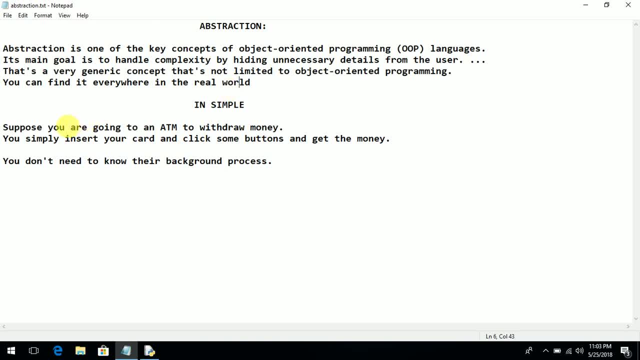 going on on the back end. Here is a simple example you can say: suppose you are going to an ATM to withdraw money. You simply insert your card and click some button and get the money. Okay, You don't need to know the background process. Simple abstraction concept is that user gives input and you have to show. 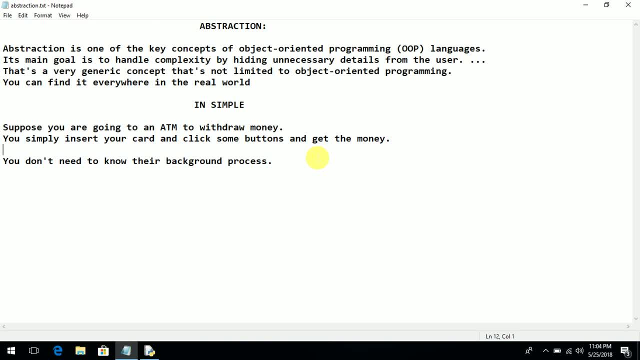 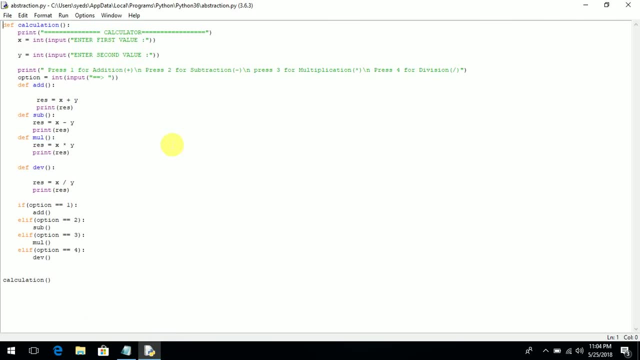 their output according to their input value. You don't need to give and user don't need to know about their background process. So how can you show this type of process in your program? So here is some simple process code example. I have made a calculator which perform addition subtraction. 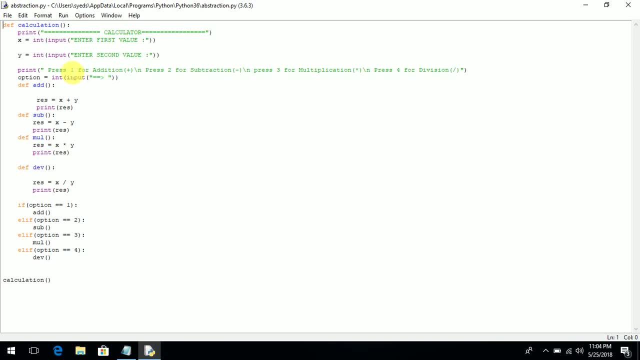 multiplication and division. so here is a simple code, here is a simple function that called calculation. there is a statement of calculator and here is two variable, X and Y. in two variable I will take input from user like enter first value, enter second value. and here is the manual, like press 1 for addition: press 2. 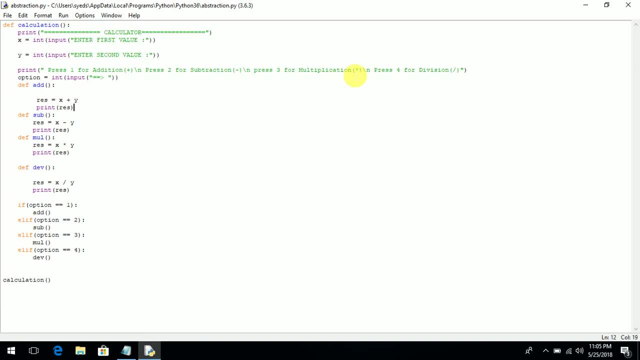 for subtraction and press 3 for multiplication and press 4 for division. and here are four different function: for first, one for addition, like simple add two values, and second one for subtraction, simple subtract two values. third for multiplication and third for addition, simple multiplication. and third for for division, and simply division between two. 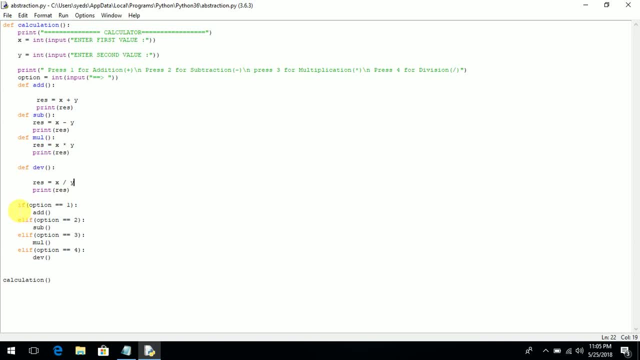 values. okay, and here is a elf elif index statement: if user press 1, so you can activate add function, and if user press 2, then activate subtract method. if user press 3, then activate multiplication method, and if user press 4, then activate division Ed green. and if user press 4, it will change the portion, so don't worry. 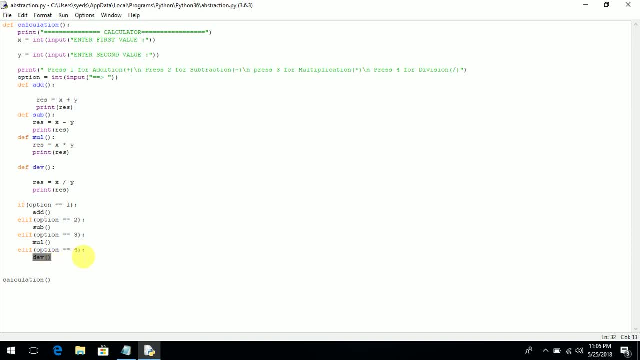 that's okay. this is my background process: what actually the user see and perform the operation on it. that is when I will run this program. first of all, you have to save this file and then this file: look, this is the actual window that user can see: big man. 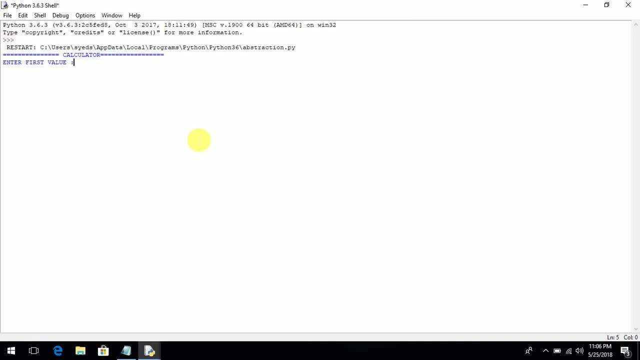 they cannot see the background process but the actual outpatient operation. in this way should be possible, reason the function delegation. so that's why it is so easy if you store row or ingress project application model to the application, you can do that and there isn't much more activity. but you don't see in this particular environment, for example, 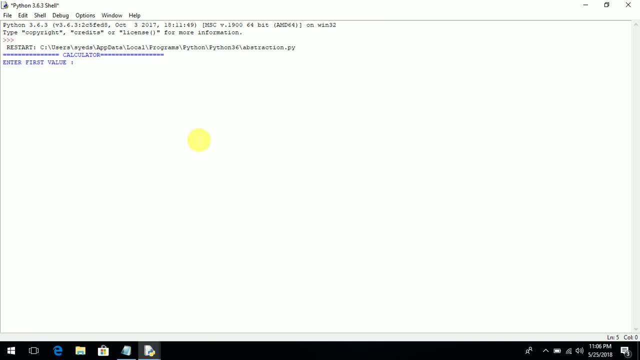 they see. first of all he or she gives input, like I'm giving. the first value is 25 and second value is 65, and after that here are some manual: press 1 for addition, press 2 for subtraction, press 3 for multiplication and press 4 for 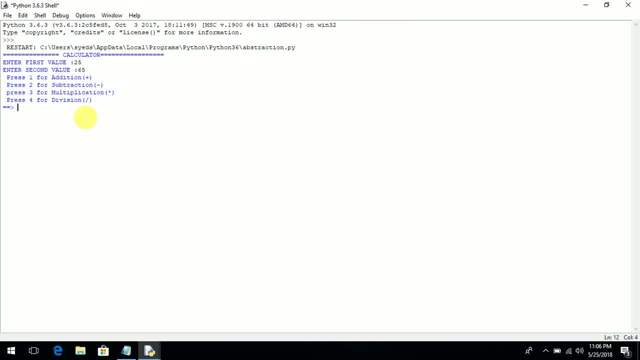 division. so I want to multiply this value. so I just press 3 and it's it give me an output 1625 when we I multiply 25 to 65. so this is the actual window. that user can interact or communicate with this window. okay, the user don't need to. 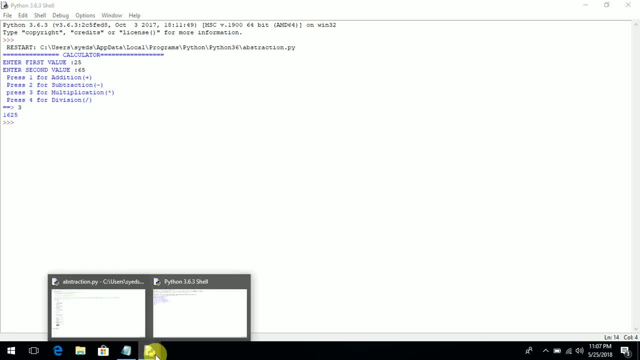 know about the background process, but I am showing you that this is the background process of this window. okay, the user only need how to in give input and how the system gives output down. the main desire of the user is to just give an output of their input. 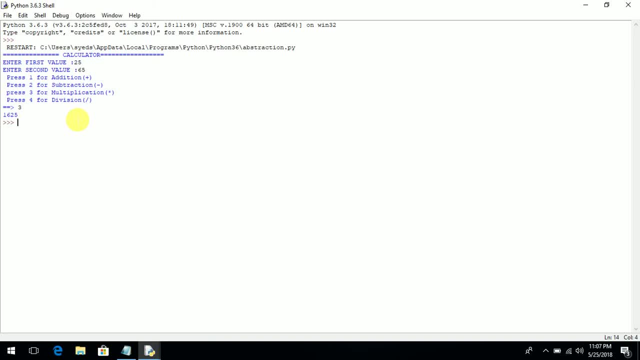 value. that is the basic concept of abstraction. you can take another example: like I am using a cell phone and I am typing some message and I know the button which I have to press for sending the message, but how the message sent to other, the person, it's none of our business. 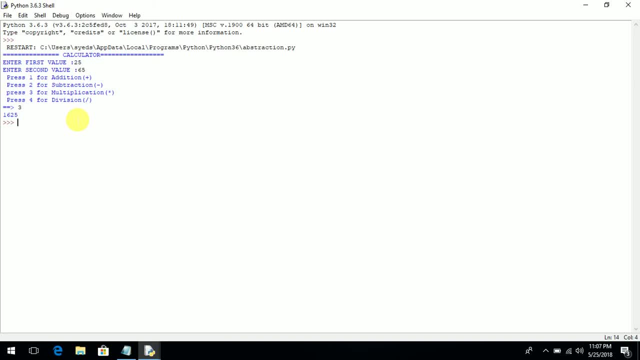 but we know the actual input and output. okay, so this is the simple concept of abstraction, hiding unnecessary detail from user. user don't need to know their background code, background process, how the work is going on, how the data display, how the multiplication and addition perform. they only need to know.